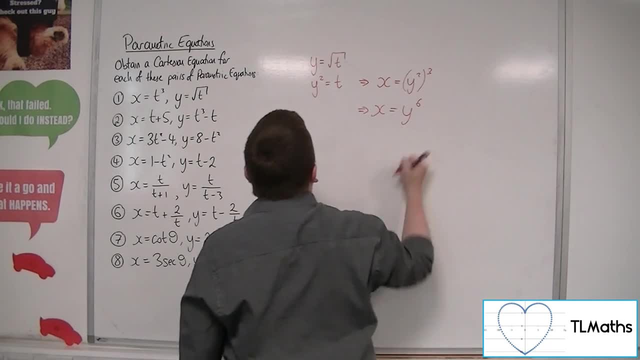 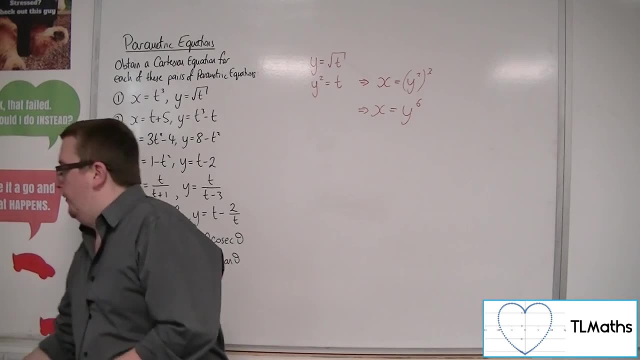 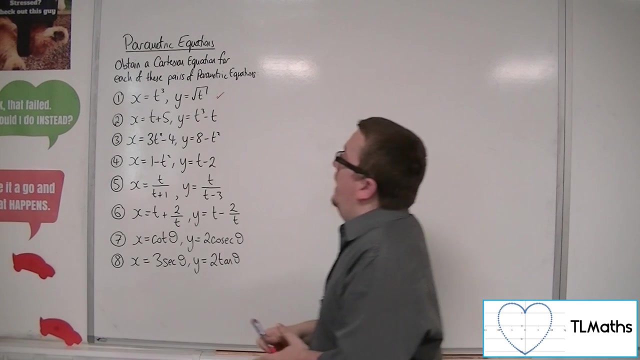 And so you could say that x is equal to y to the sixth, And there is a Cartesian equation that represents number one. Okay, so that's our first one, Right? let's have a look at number two. So x equals t plus five, y equals t cubed minus t. 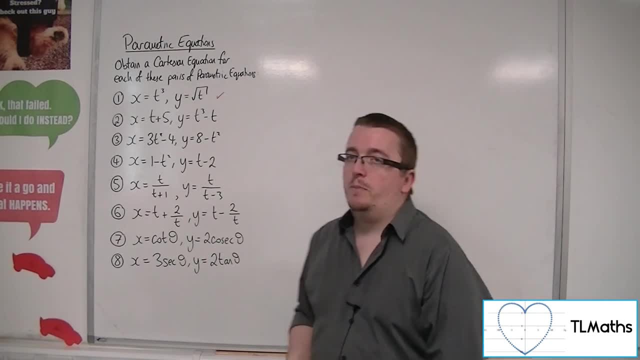 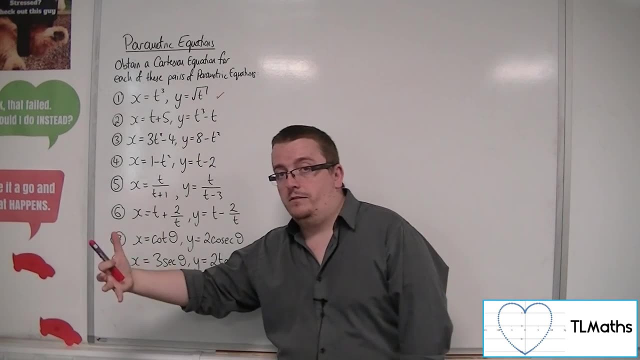 Now, in this case, if I looked at the y equals t cubed minus t, there is actually no way to get t equals something on the other side, So t equals a function of just y. Okay, there's no way to actually rearrange that, to do it. 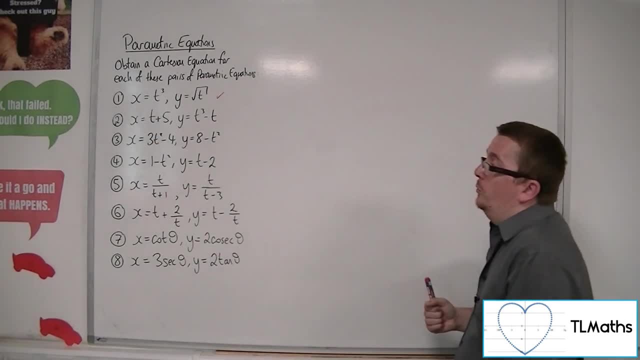 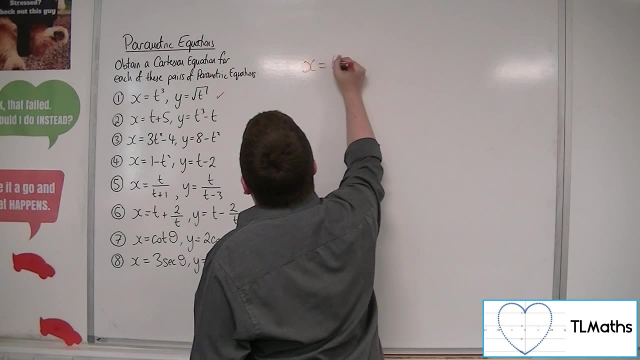 So the only one I can rearrange is the first one. the x equals t plus five. So if there was a simpler one to rearrange, go with that one. So x is equal to t plus five. So rearranging that, you can say t is equal to x minus five. 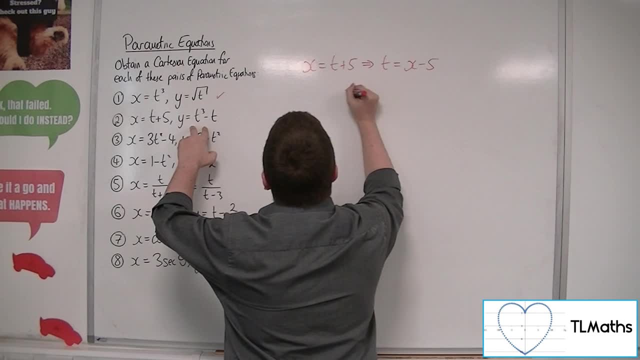 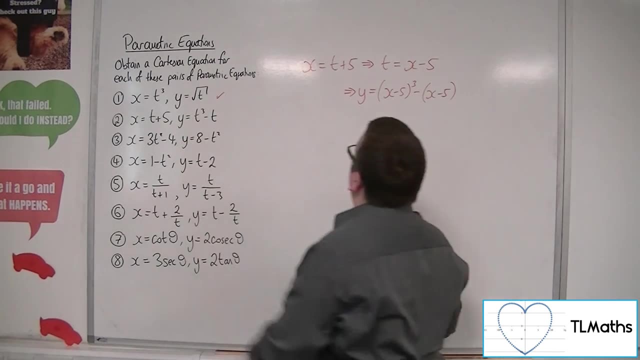 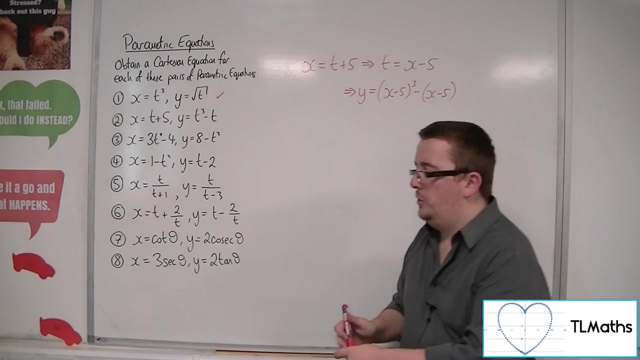 Then you can substitute that one into the second equation. So y equals x minus five, cubed minus x minus five. Okay, and that would be my Cartesian equation. Now you could expand out all those brackets. I don't think we need to, okay, but that's where we would be at. 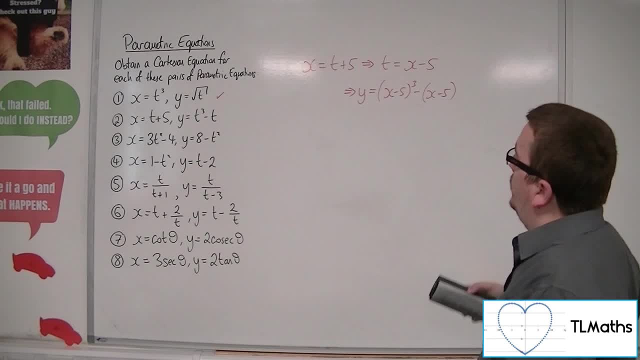 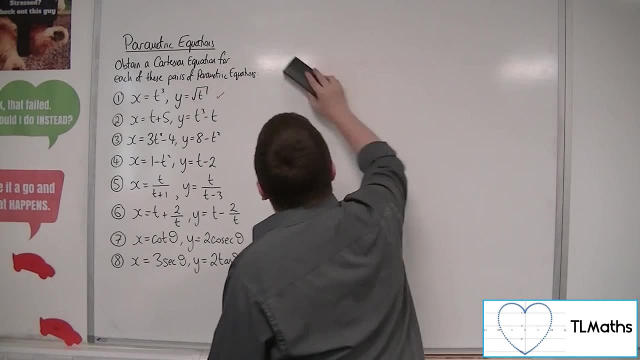 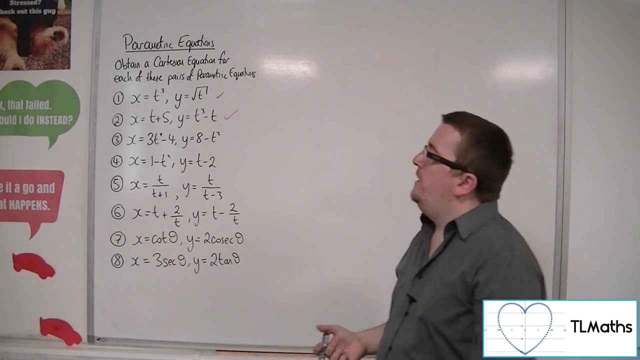 Okay, So it might be that the question might ask you to write it in a particular format, but otherwise that's fine. So that's number two, All right. number three: x equals three t squared minus four, and y equals eight minus t squared. 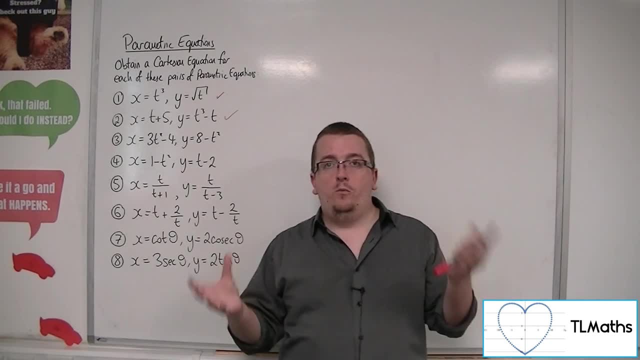 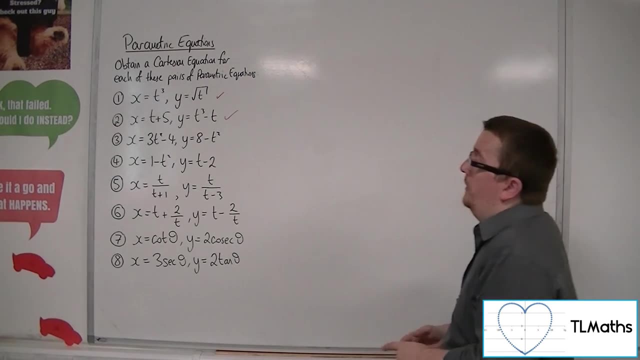 Now it can be that in certain circumstances, you might be going well. actually, I seem to have no choice here. I must get t equals, and I would need to Well in both of these cases in order to do it. 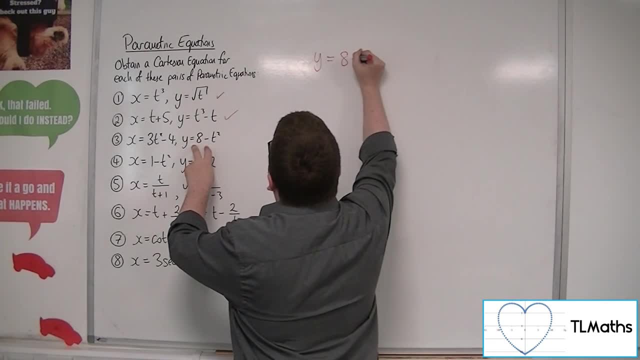 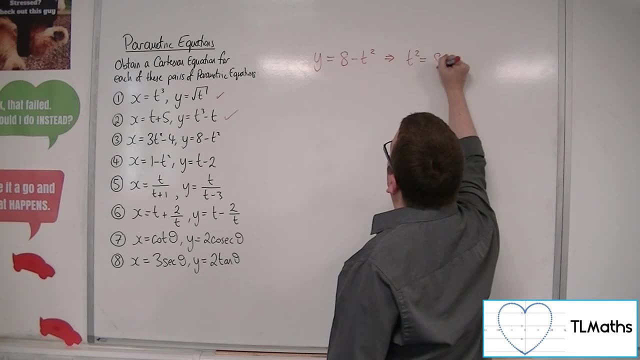 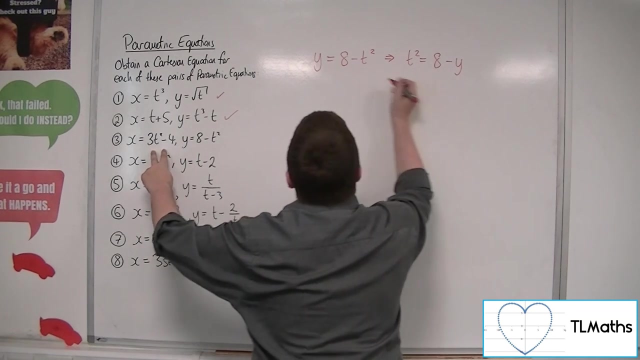 However, what might be easier to work with- and certainly is in this case- is if you take one of these equations and rearrange it to get t squared, And then you can replace the t squared in this equation with this one, So that means that x is equal to three lots of t squared. 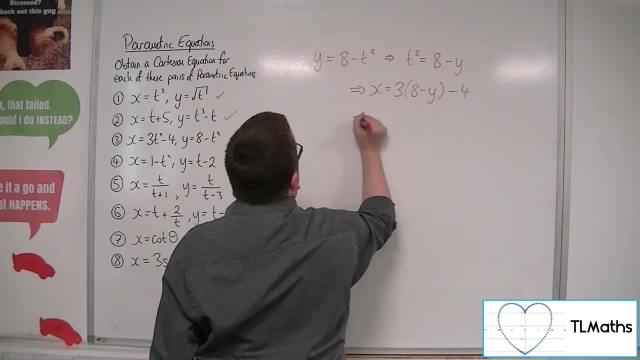 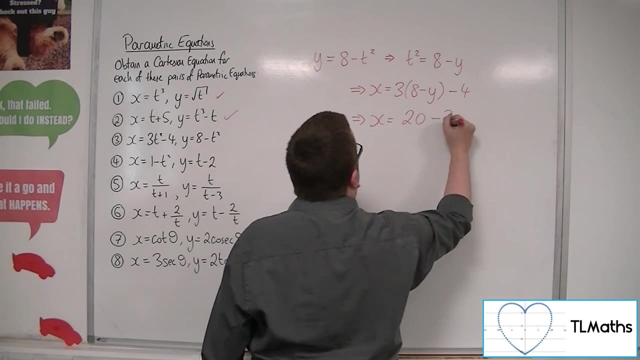 So three lots of eight minus y take away four, And so if we tidy that up, If we add up, we get three. eights are twenty-four. take away four, so twenty take away three y, And there's a Cartesian equation that represents number three. 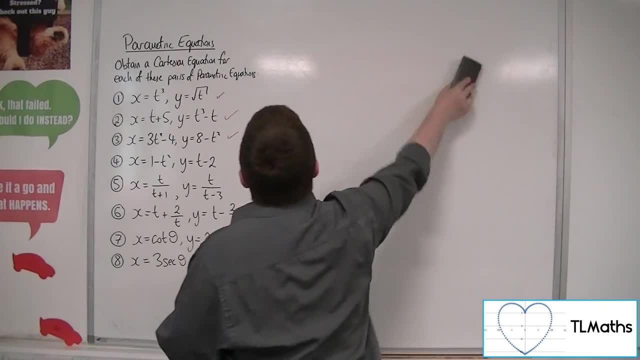 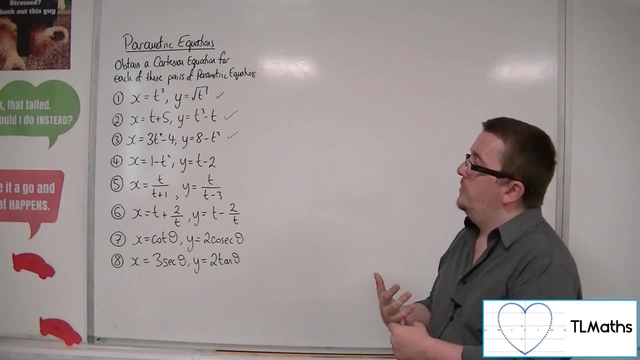 Okay, So you're seeing there's a few tricks of the trade here to keep an eye on. Now number four I've included just as another reiteration of this: Well, I could rearrange x And do it this way. 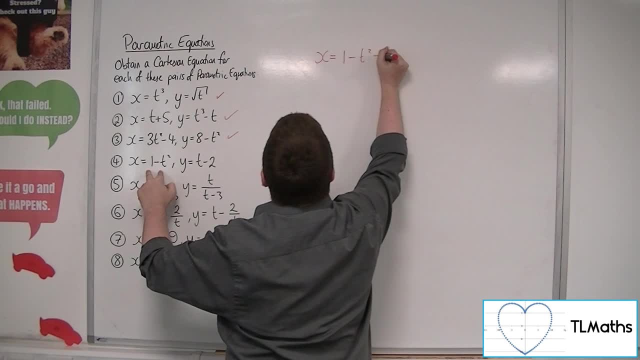 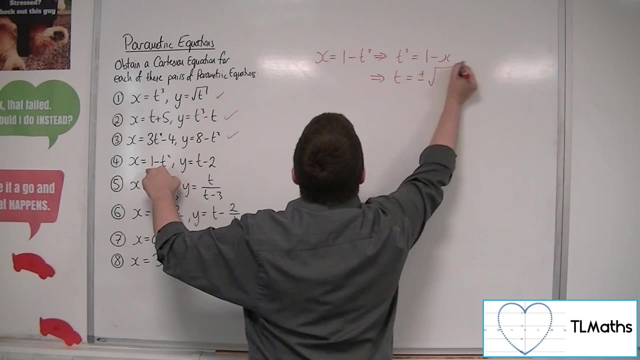 So you could say to yourself: well, x equals one minus t, squared rearranges to t. squared is equal to one minus x, And then you'd have to square root both sides, which brings in a plus, minus, And then I'd have to substitute that into the y. 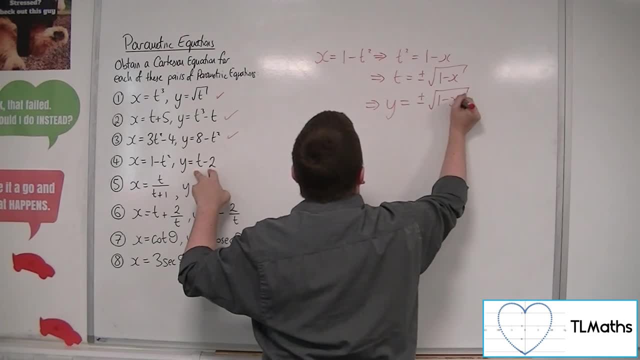 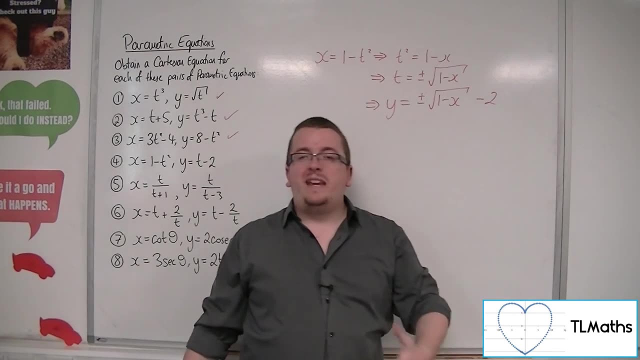 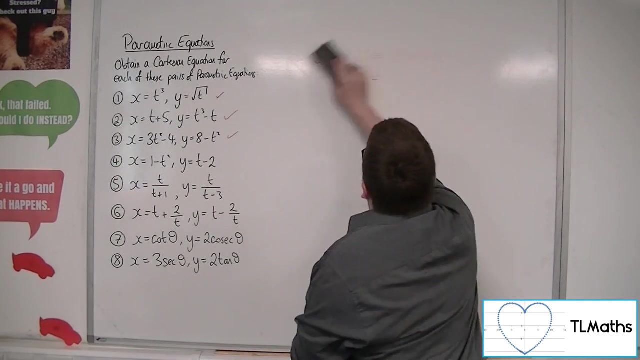 Now, this isn't wrong, but it's messy, as you can see. Okay, The fact that it is messy means that I don't particularly want to have To deal with that. I don't want to have to use that, So it might be easier to do it the other way round. 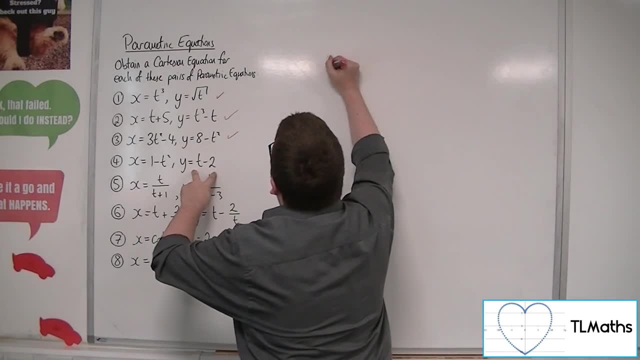 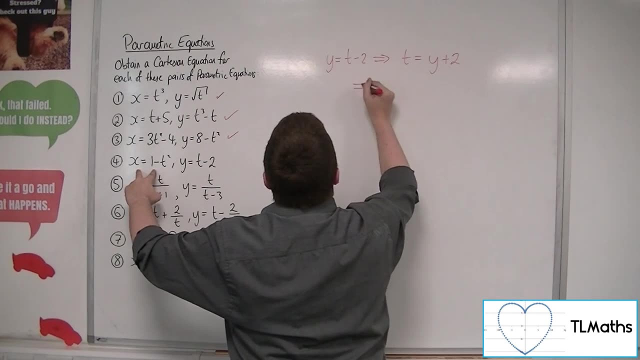 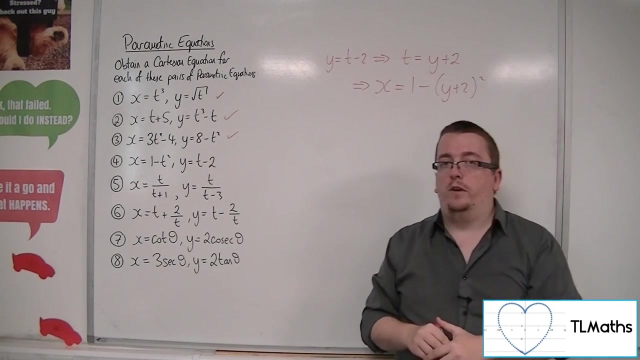 So instead, if I take the y equals t minus two and rearrange that to get t is equal to y plus two. I can then substitute that into the other equation And I get something that's much easier to work with. Okay. 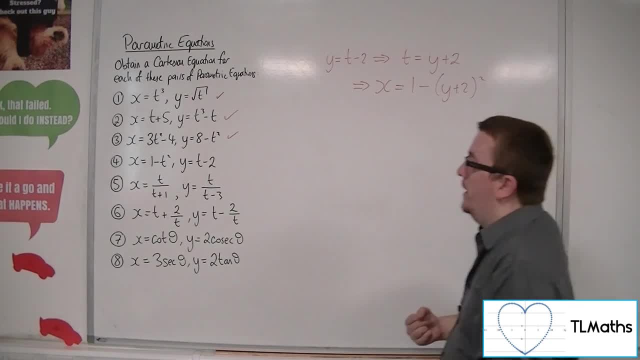 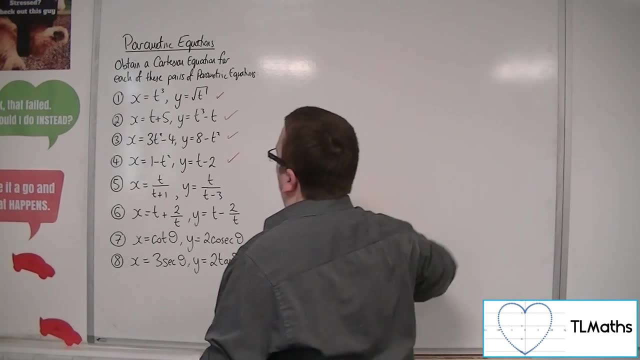 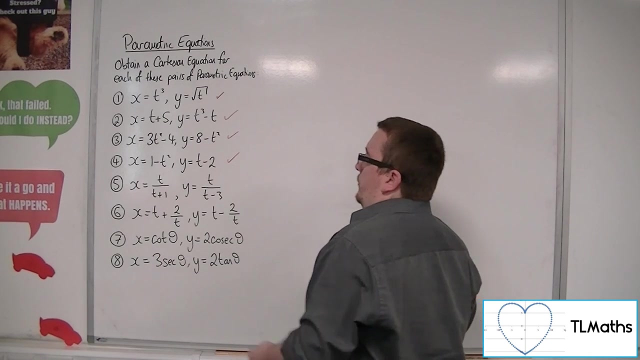 I don't have the plus minus, I don't have the square root. Okay, So that's number four. Now, sometimes, as with number five, the algebra can get a little bit intensive. Okay, So, looking at either of these, neither of those look easier than the other. 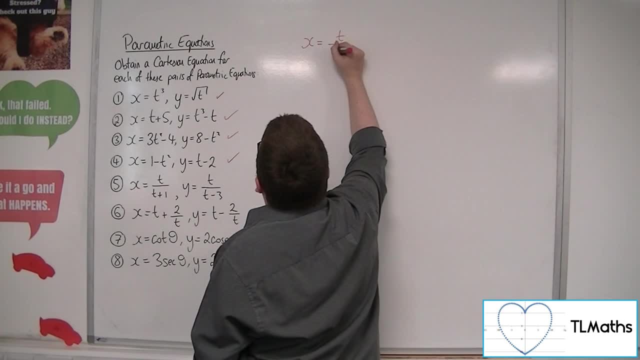 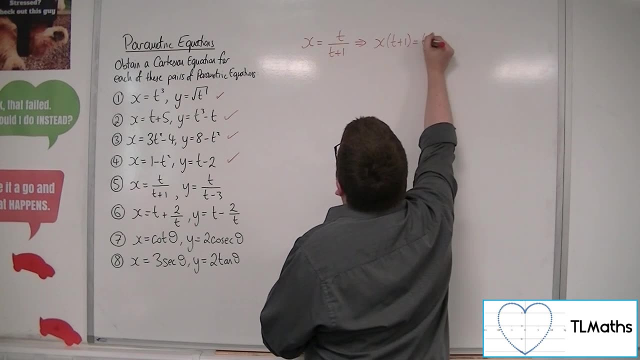 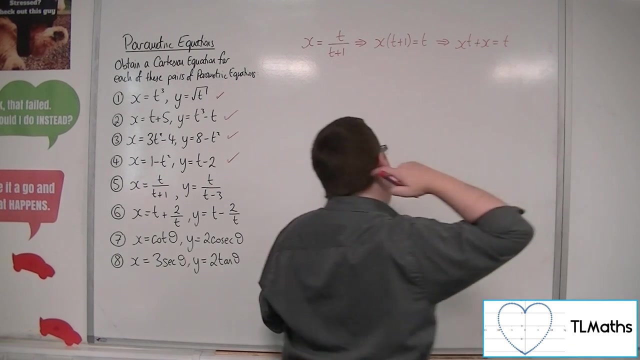 So probably best to just choose one and see where we go with it. So I'm going to multiply both sides by the t plus one. I'm going to have to expand that, I'm going to expand that left-hand side, And now I need to isolate the t. 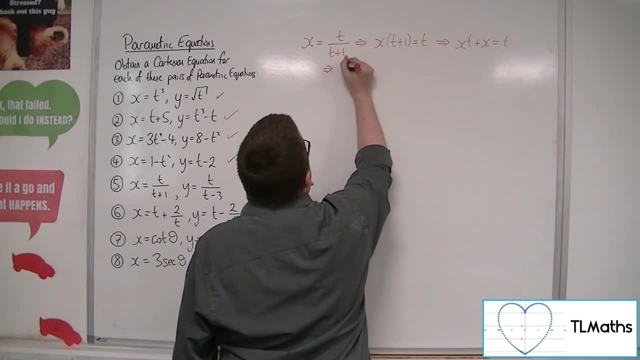 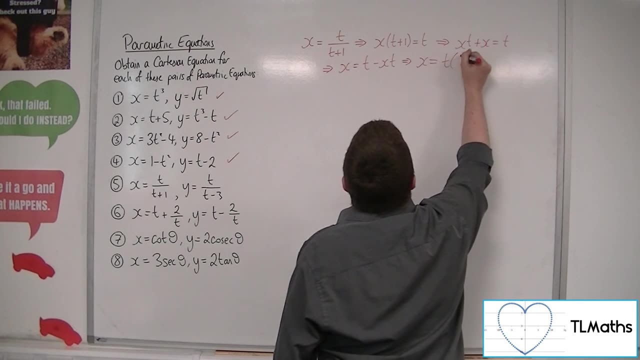 So if I take the x- t over to the other side, I'm going to get: x is equal to t minus x t Factorise the right-hand side. So bring the t outside of a bracket and have one minus x inside. 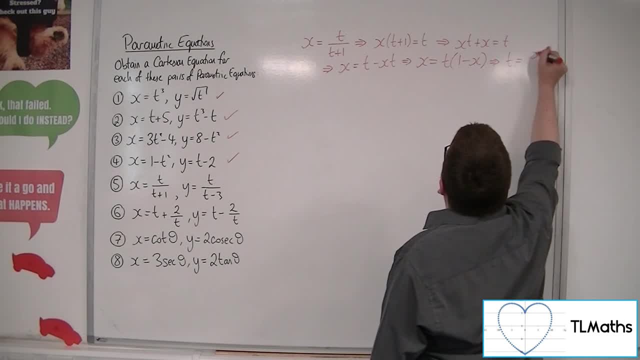 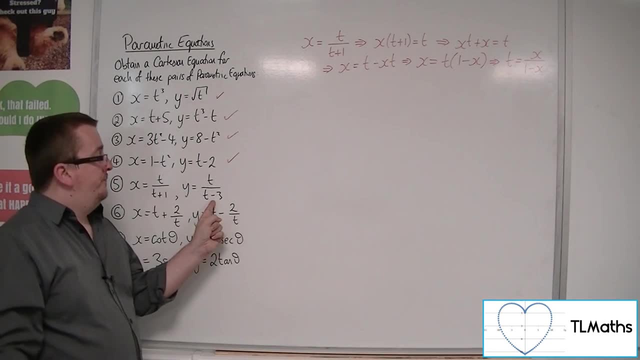 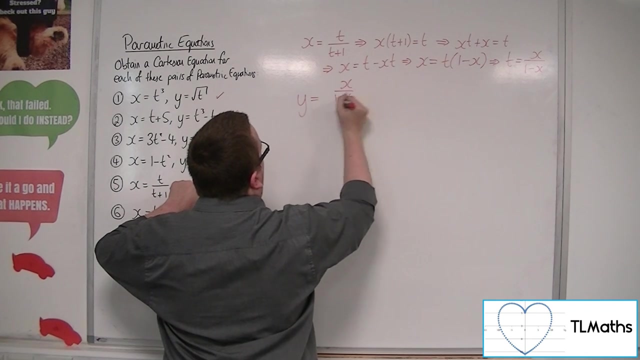 And then I can rearrange to get t equals x over one minus x. So I can now substitute that into the other equation, Into the second equation. So y is equal to t, So x over one minus x over t. 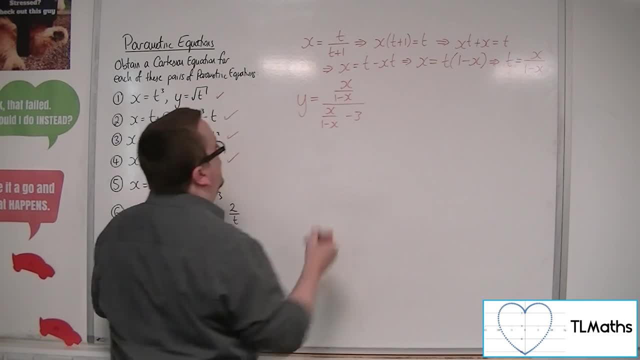 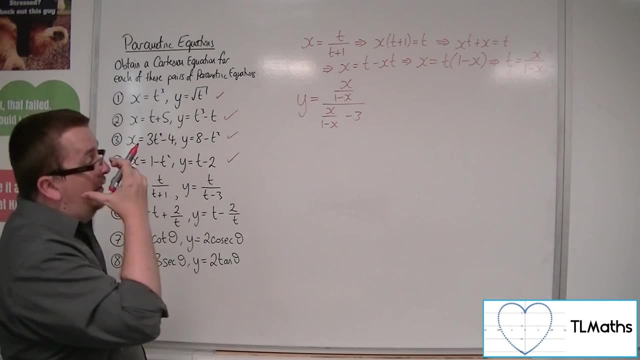 So x over one minus x, take away three. Now this is a Cartesian equation, but it is absolutely ghastly having fractions within fractions. So if I multiply top and bottom of this fraction by one minus x, I'm not changing the size of the fraction at all. 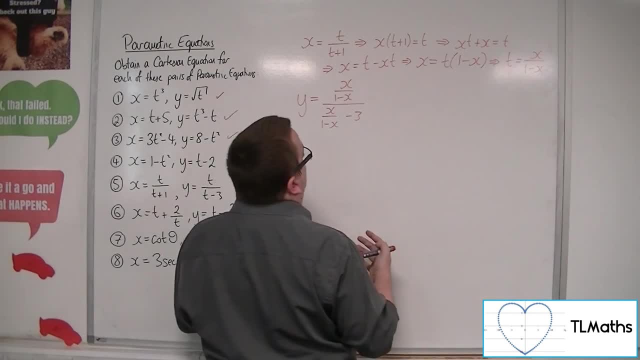 But if I multiply top and bottom of this fraction by one minus x, I'm not changing the size of the fraction at all. But what I will do is I will get rid of the denominators. So if I times the top the numerator by one minus x, I just get x. 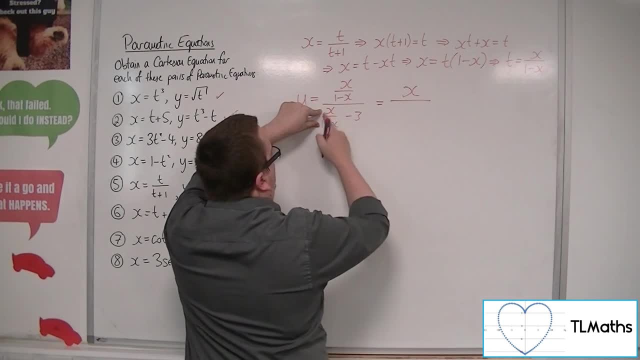 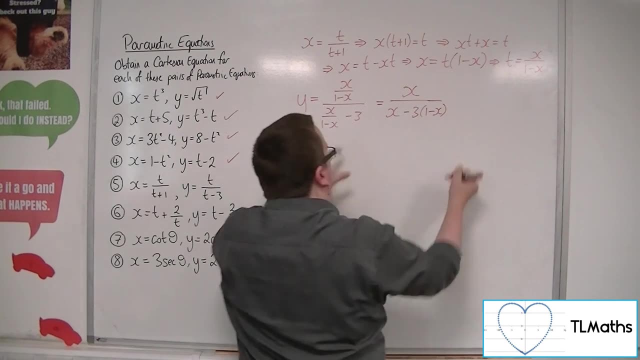 If I multiply the denominator by one minus x, I just get x there. Then take away three lots of one minus x. So let's tidy that up. I've got x in the numerator. I've got x minus three plus three x in the denominator. 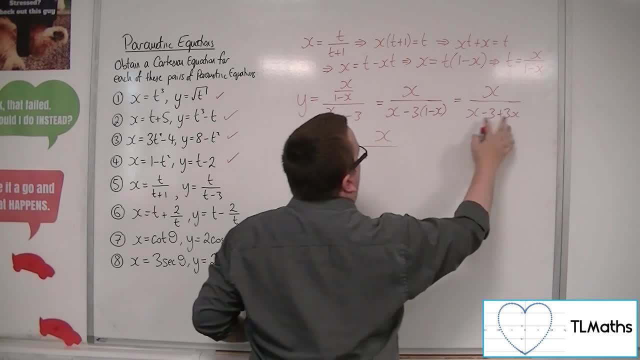 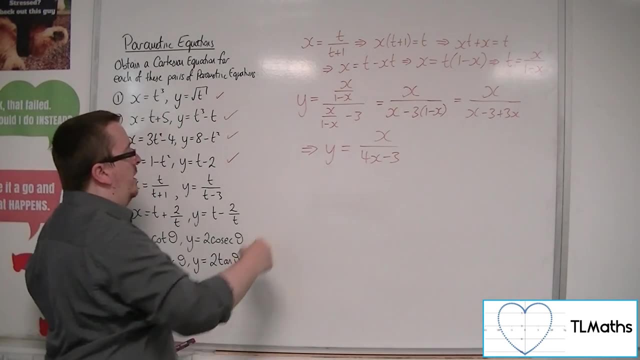 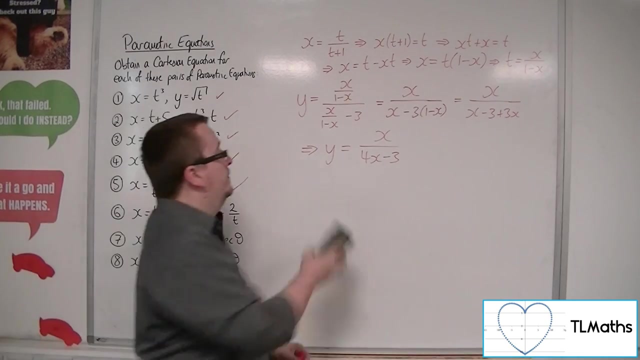 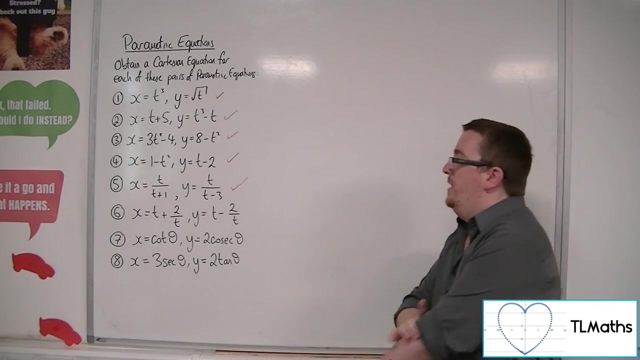 So y is equal to t, So y is equal to t, So y is equal to x over four, x minus three. Okay, and that's much more tidy. And there is my Cartesian equation that represents number five. Now number six. 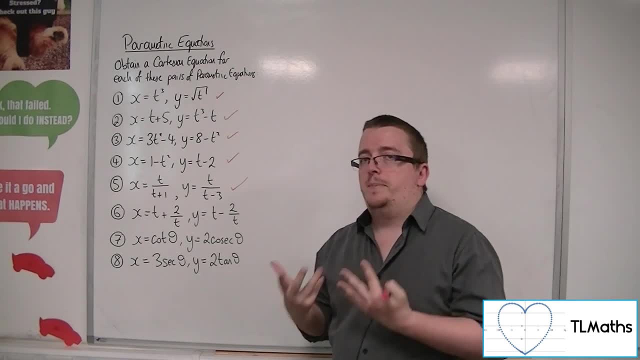 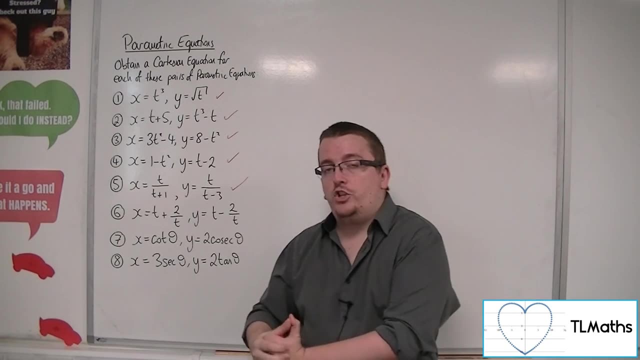 Number six looks like it's going to be trouble, And the problem is that it's going to be trouble. The problem with number six is that neither x or y rearrange to get t equals Okay, so in other words, I've got a problem. 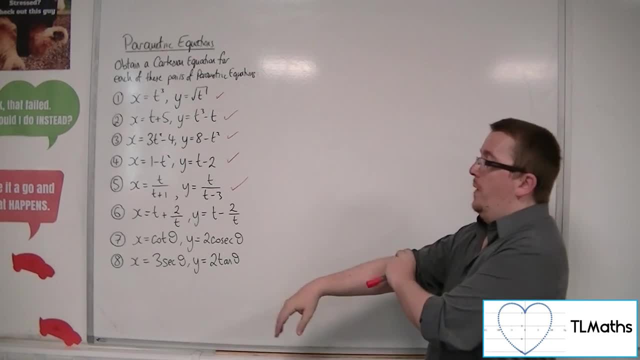 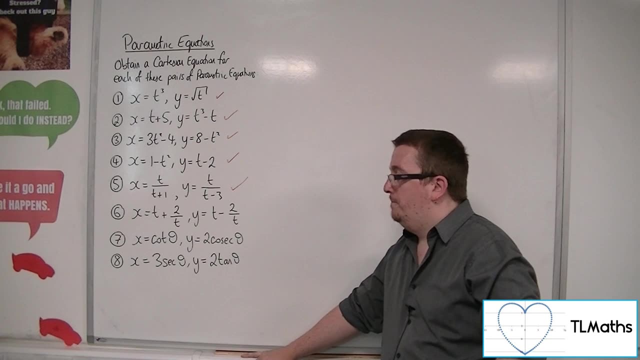 And nine times out of ten, if you were in this situation and you couldn't rearrange either, that probably means that you can't get a Cartesian equation. However, with this one you can, Because if you notice that actually you've got. 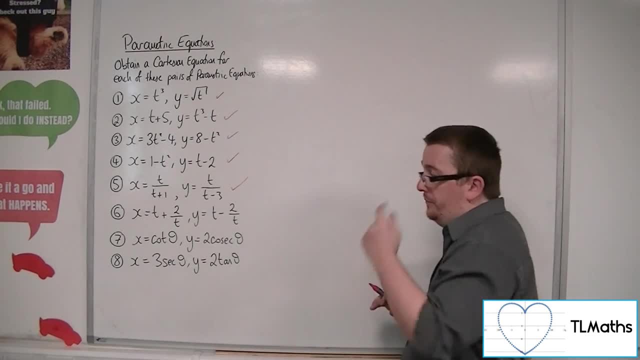 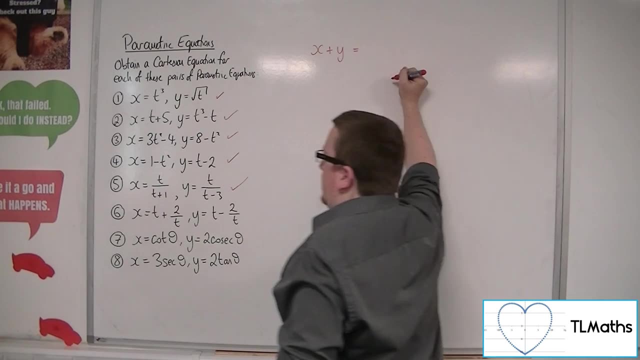 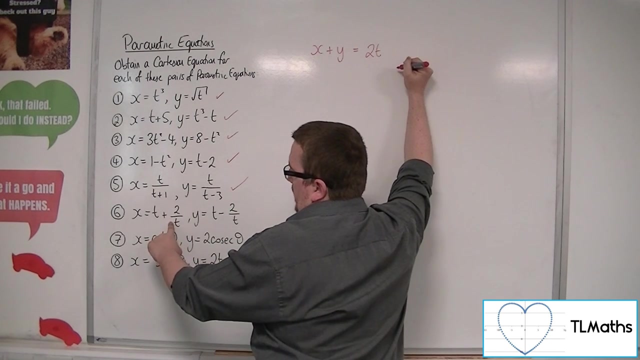 The same two elements, but one is plus, one is minus. Then what you can think about is: well, if I add the x and the y together, I'm going to get t plus t, so two t, And I'm going to have two over t, plus negative minus two over t. 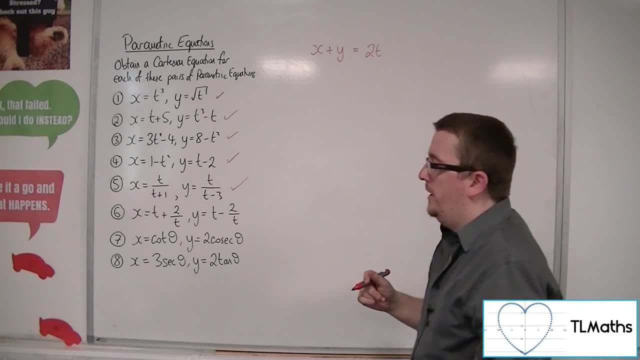 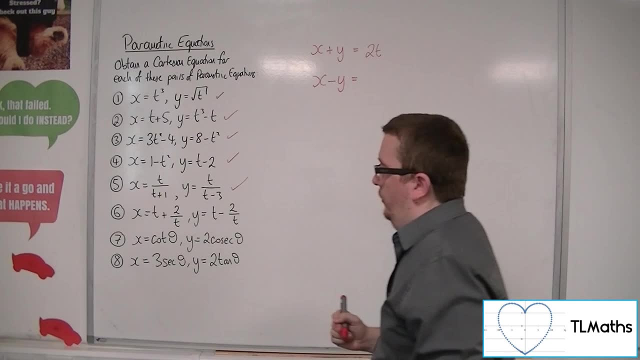 So they cancel each other out. So x plus y is equal to two t, And if I also find out what x minus Minus y is equal to, So I'm going to get t. take away t, so that's zero. 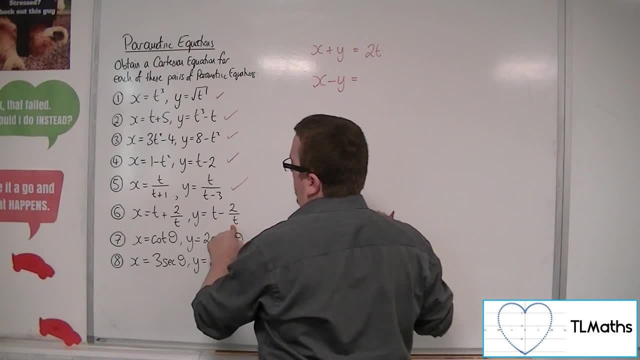 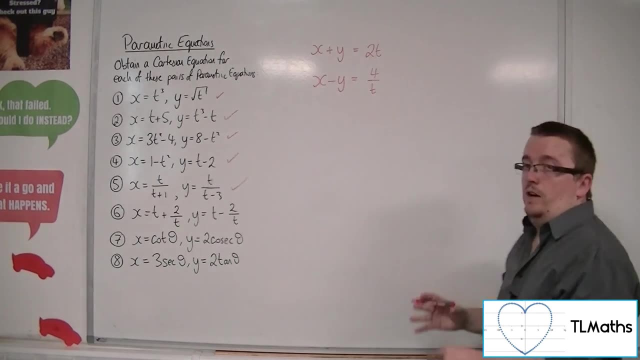 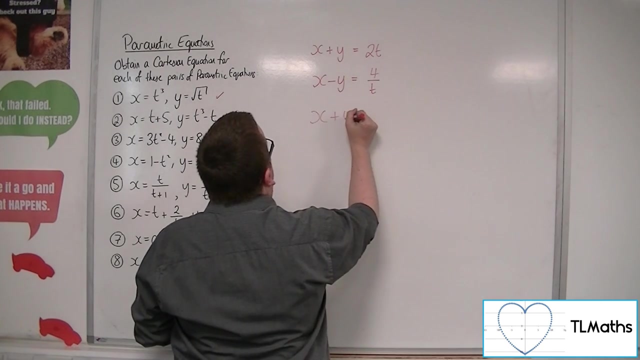 Two over t. take away minus two over t is two over t plus two over t, So that's four over t. And now if I multiply these two equations together, I will cancel the t's out, So I'll get x plus y times x minus y is equal to two t times four over t. 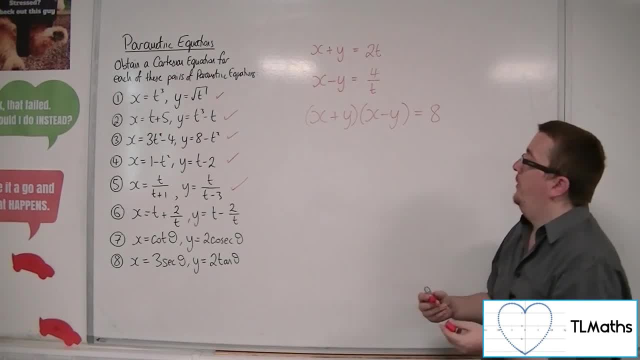 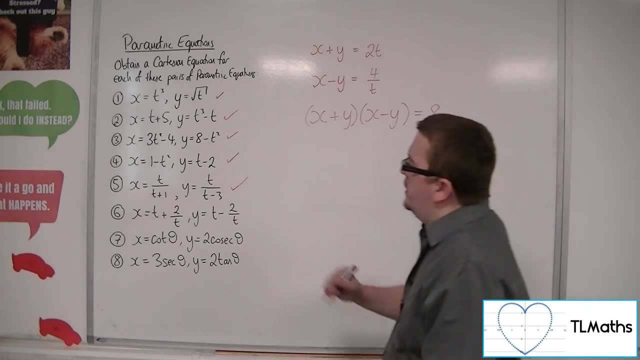 which is just eight, And I now have a Cartesian equation that represents number six. Now you might be looking at that going. well, how on earth would you initially spot that? And you know, fair credit, that it is quite a tough one to spot, okay. 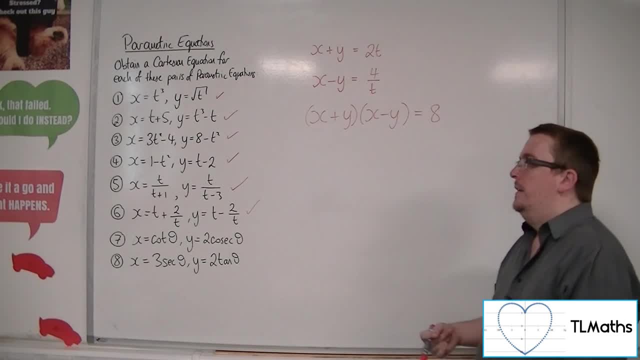 It's not one that you wouldn't, you'd really be looking out for In some cases where these kind of questions have come up, In some cases where these kind of questions have come up previously in exams. they've given you a hint. 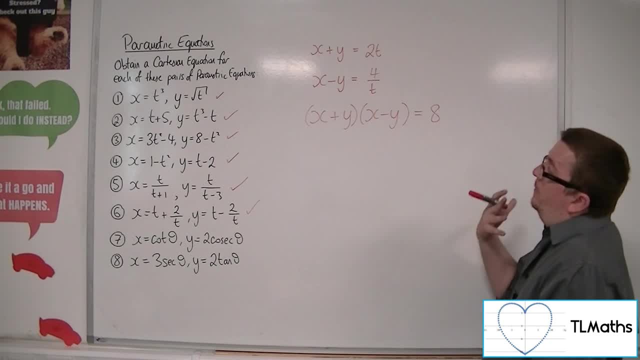 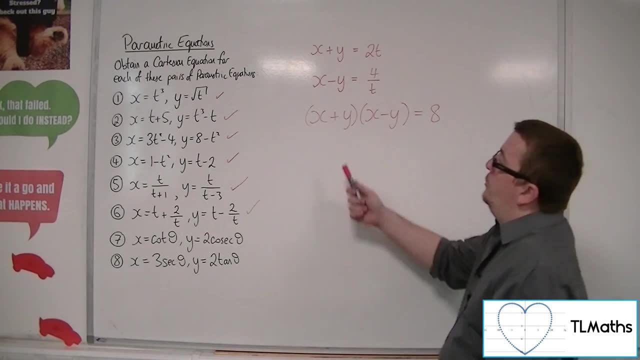 It's either in the case of: by finding x plus y and x minus y, show that you can write the Cartesian equation as: x plus y, x minus y equals k and you need to calculate k. So there have been questions that have involved that type of problem before. 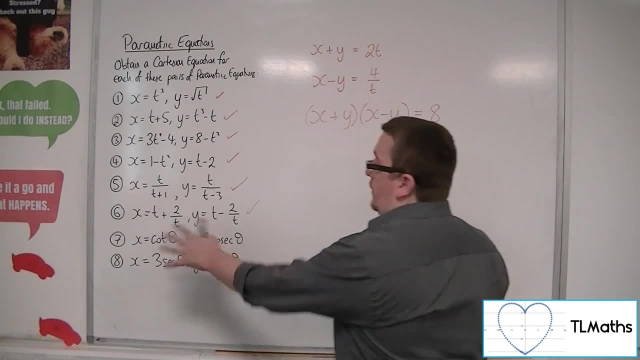 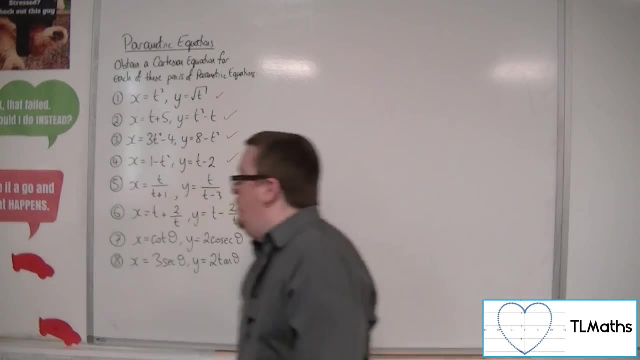 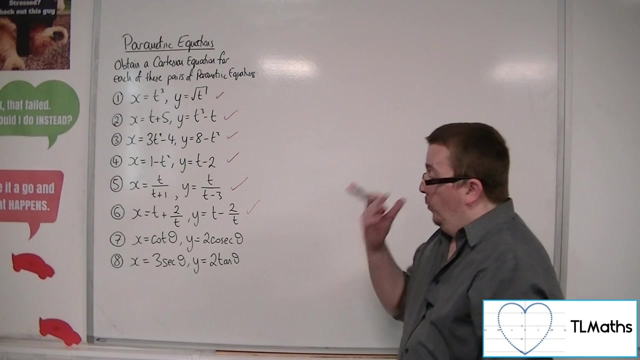 But not necessarily as like do this from scratch. okay, Now, when you get onto questions like number seven and number eight and you're dealing with these trig functions, what you really need to do is remember what trig identities you have. 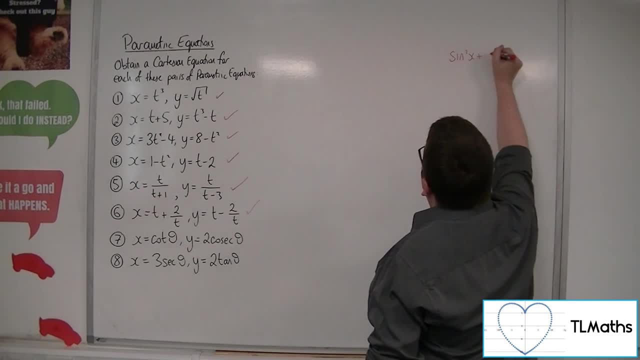 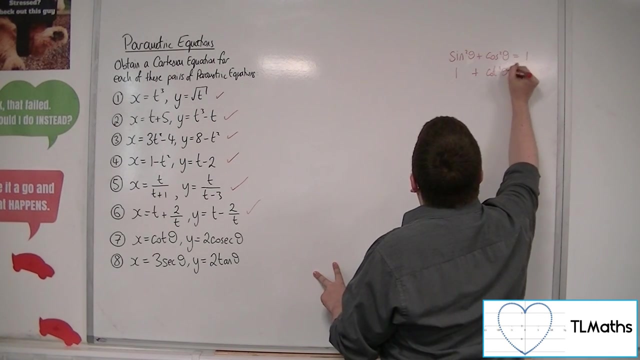 Now remember, we've got the sine squared plus cos squared is one, Okay, Or theta. if we go with theta Now, if you divide both sides by sine squared, you get one plus cot squared theta is equal to cosec squared theta. 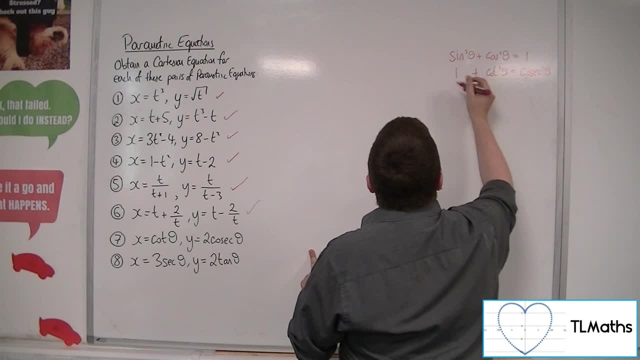 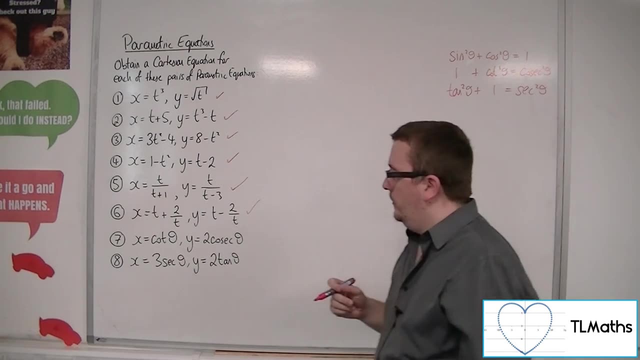 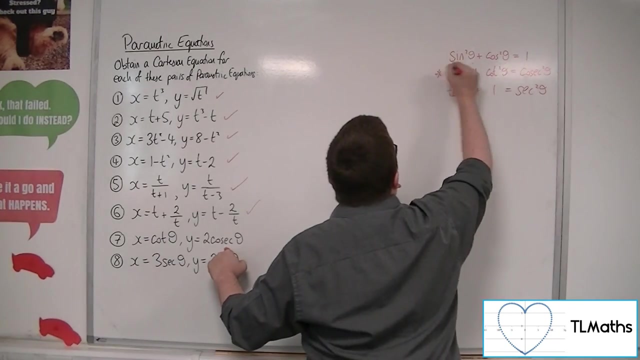 And if you divide the original equation by cos squared, you get tan squared theta, plus one is sec squared theta. So if we have a look at number seven here we've got cot and cosec, Which fits into this one here. So we know that cot theta is x. 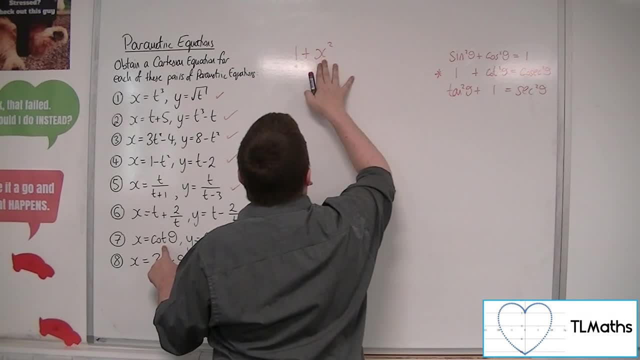 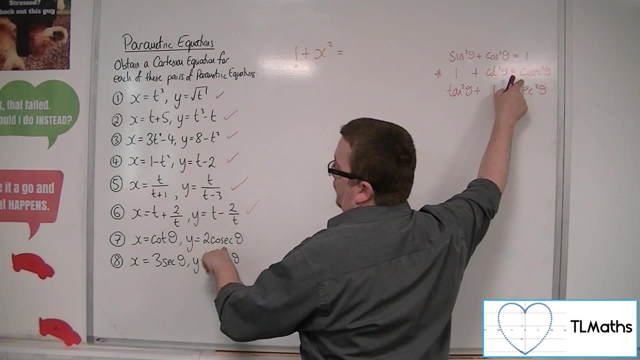 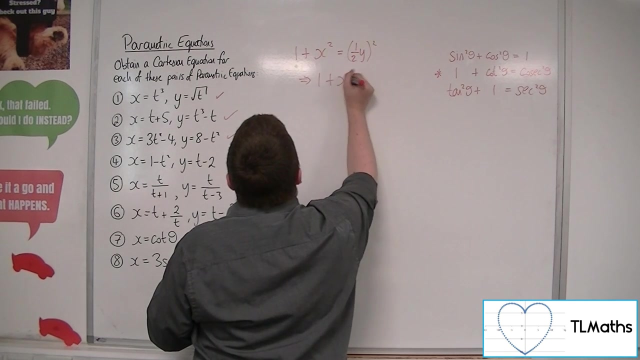 So we could say: one plus x squared, one plus cot squared is equal to cosec squared, And cosec theta would be y over two, halving both sides. So that would be one half y squared. So you could write that as one plus x squared is equal to a quarter y squared. 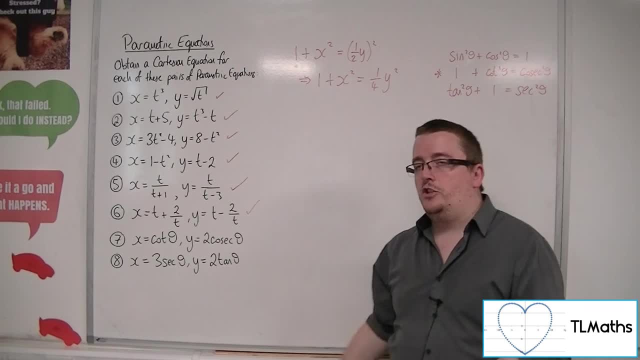 And that would be your Cartesian equation that matches those parametric equations. So if you spot parametric equations that involve trigonometric functions that fit nicely into any of these identities, then we can use those identities for substituting in. So that's number seven. 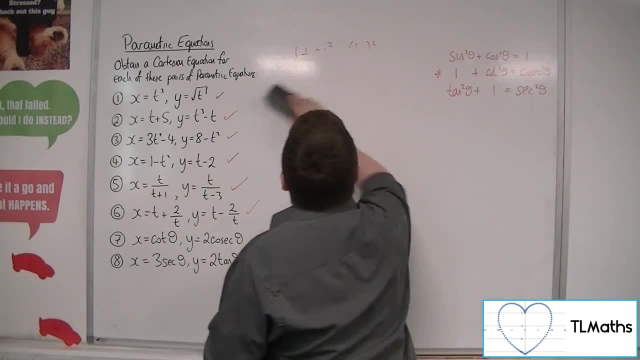 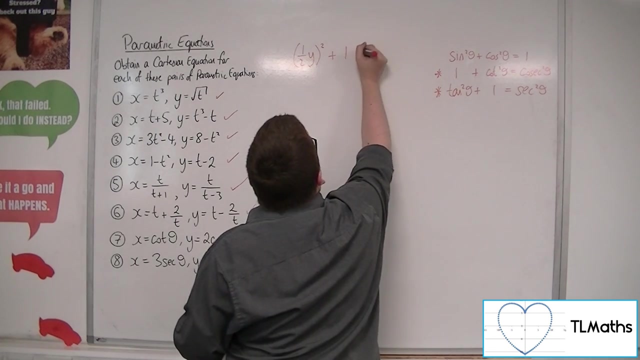 And number eight works in a very similar way, Because now you've got sec theta and tan theta, So it works with that identity. So tan squared, which is y over two, So a half y squared plus one, is equal to sec squared. 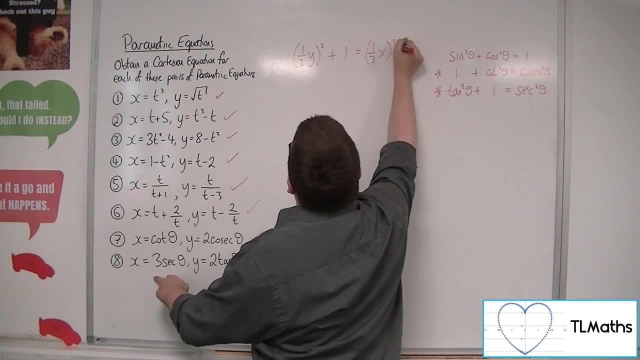 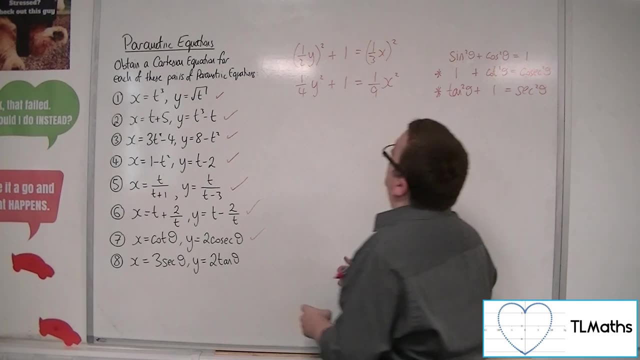 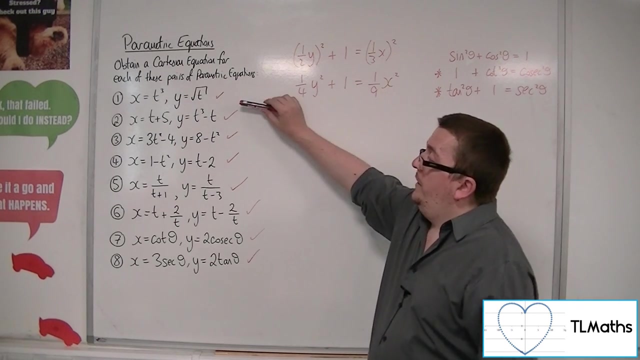 which is one third x. So one third x squared. So that would be a quarter y squared plus one is equal to a ninth x squared, And there is your Cartesian equation for number eight. So in a lot of cases, in those first five, 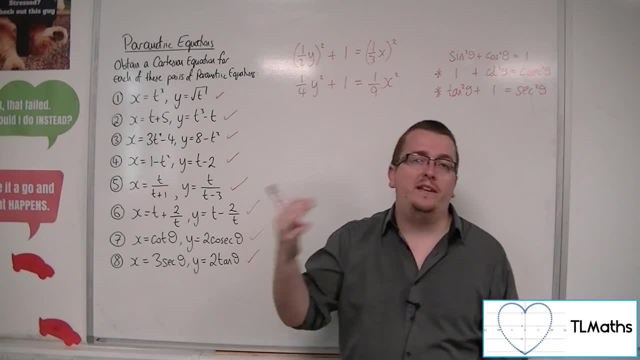 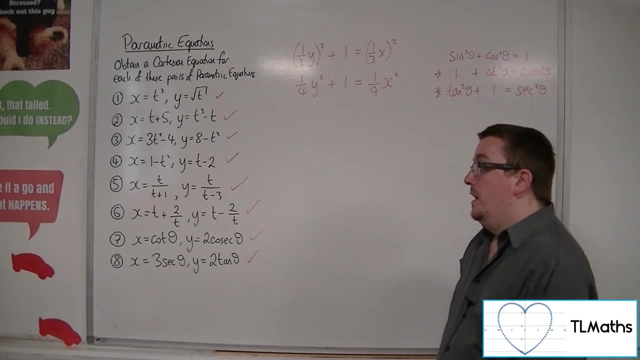 we were looking at rearranging one of the equations, substituting it into the other. It doesn't matter whether you end up with x equals or y equals at the end, It doesn't matter at all. Number six: we had to use a trick. 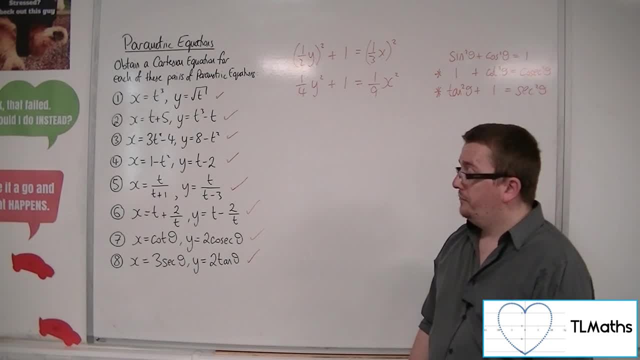 Adding and subtracting the two equations and multiplying them together. In questions seven and eight we had to revert to trigonometric identities.